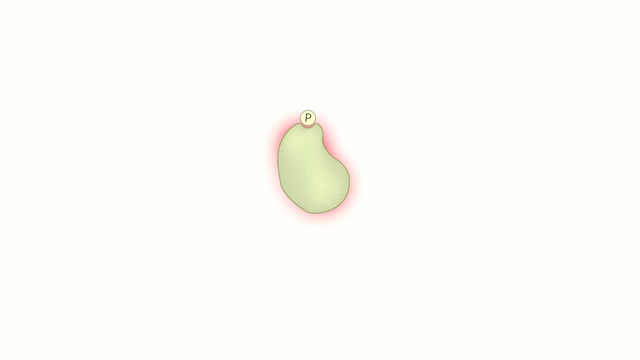 We previously mentioned that phosphorylation leads to the activation of a protein. However, this describes only one out of three possible effects. First, the protein may become activated. Second, the protein may be deactivated. Third, the transferred phosphate group can be a signal to other proteins. 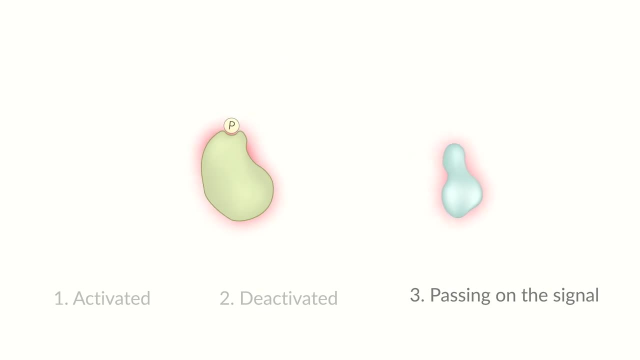 to interact with the target, thereby passing the signal on. Have you ever wondered how the signal is switched off? Another group of enzymes, the phosphatases, are able to remove the phosphate group from the target. protein Phosphorylation is therefore a reversible. 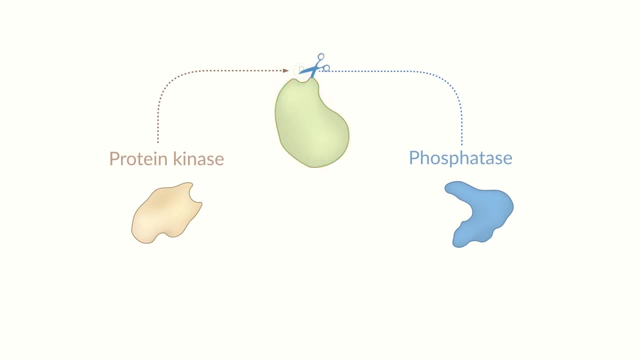 protein modification that is regulated by a balance of kinase and phosphatase activity. As you can see, signal transduction through the addition of phosphate groups is a powerful mechanism. Accordingly, the enzymes are kinases with the prefex "-kine-", as in kinetics. 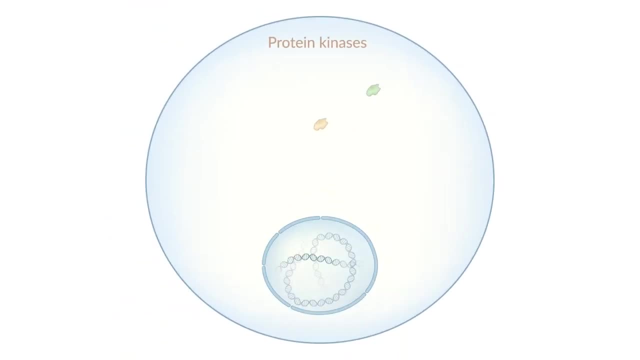 meaning to move. Protein kinases are driving forces for many cellular processes and more than 500 different protein kinases have been identified. All kinases are essential or have to be� важedk for properification. If there is nowhere to go, victims must be washed off the subject, and there is no waiting in any flamBC dropping supplies to the差аz. osTM finish working, songanian m international or in another research study about this kind. 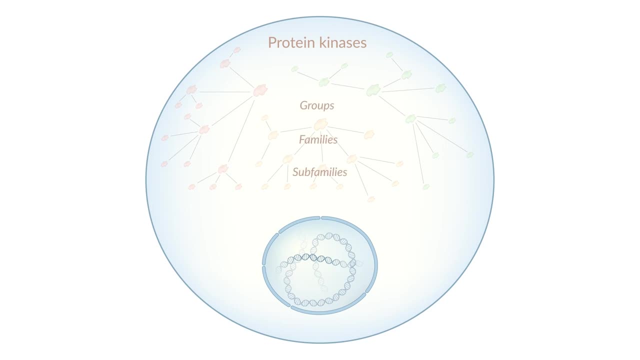 into a fairly complex system of different groups, families and subfamilies. This classification takes into account both structure and function. Given the large number of kinases, it is impossible to remember them all. However, you may want to keep in mind that they can be broadly classified. 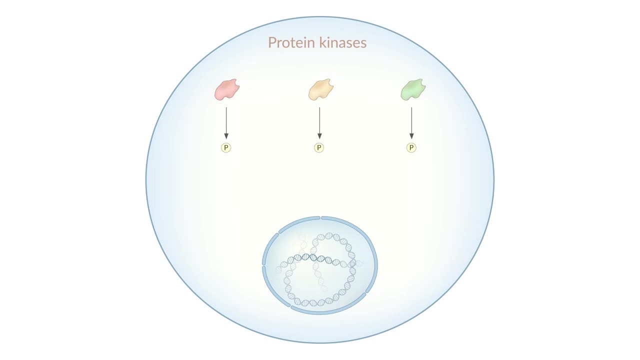 according to the amino acid residues they phosphorylate. They usually act on one of three residues: tyrosine, serine or threonine. However, this comes with a twist: Kinases that are able to transfer phosphate groups to serine residues. 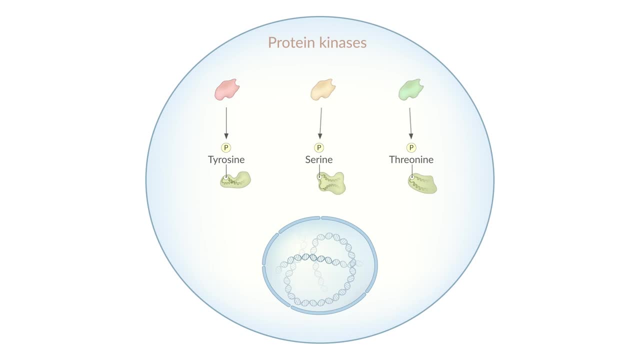 are also able to do so for threonine residues. Therefore, they are often grouped together as serine-threonine kinases. This leaves us with two large groups: tyrosine kinases and serine-threonine kinases. Regardless of the amino acid residue, that is, phosphorylated. 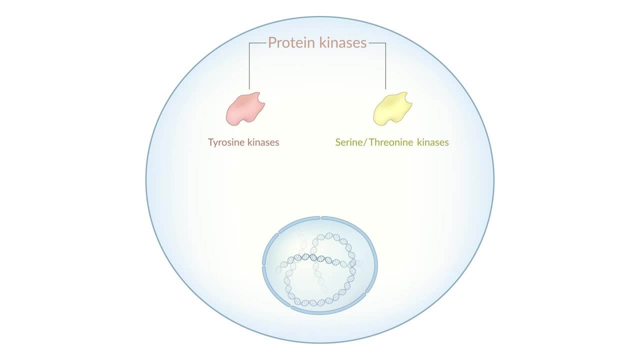